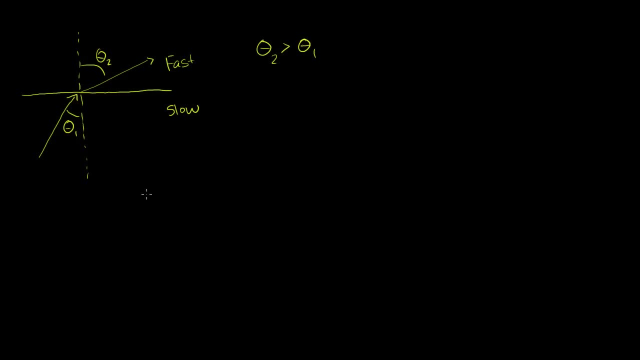 we get, theta two is going to be greater than is going to be greater than theta one. Now what I want to ask, or what I want to figure out in this video, is is there, is there some angle depending on the two substances that the light travels in? 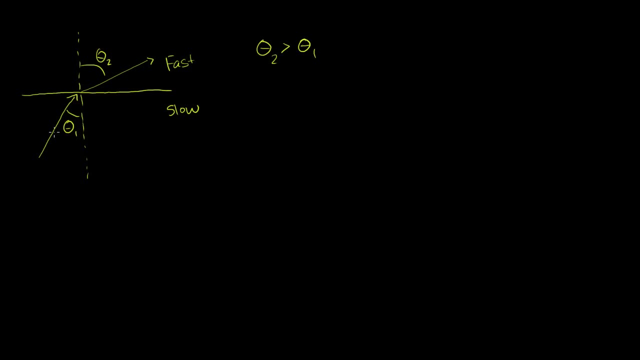 where, if this angle is big enough- because we know that this angle is always larger than this angle, that the refraction angle is always bigger than the incident angle moving from a slow to a fast medium- is there some angle? if I were to approach it right over here, 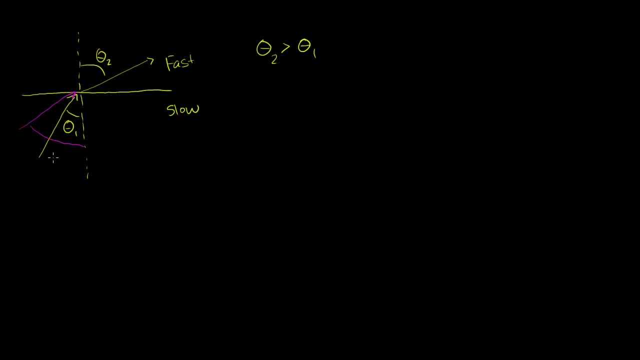 if I were to approach at this angle. let's just call this, let's just call this theta three. is there some angle theta three where that is, that is large enough that the refracted angle is going to be 90 degrees? 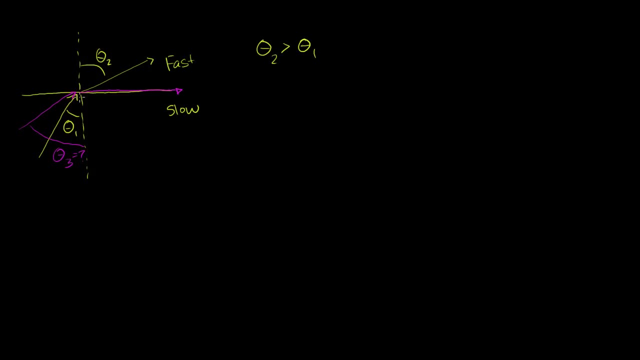 if that light is actually never going to escape into the fast medium And if I had an incident angle larger than that. so if I had an incident angle larger than theta three. so let's say I had an incident angle like that and so, whatever that is, 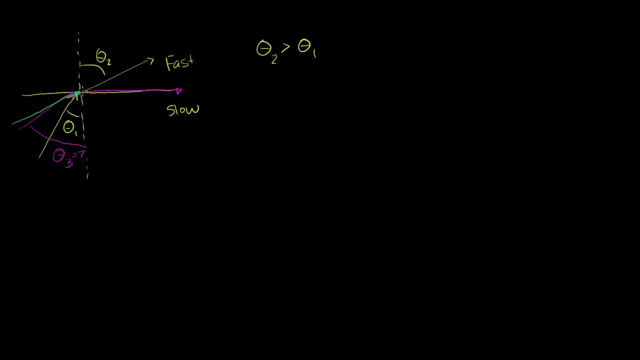 that it actually that the light won't actually even travel along the surface. it definitely won't escape, it won't even travel along the surface, but it'll actually reflect back. So you actually have something called total internal reflection. And to figure that out, 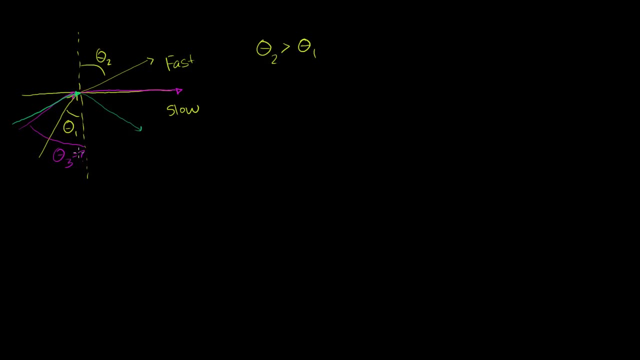 what we need to do is figure out at what angle- what angle- theta three- do we have a refraction angle of 90 degrees? At what angle- theta three- do we have a refraction angle at 90 degrees? And then that angle, that incident angle. 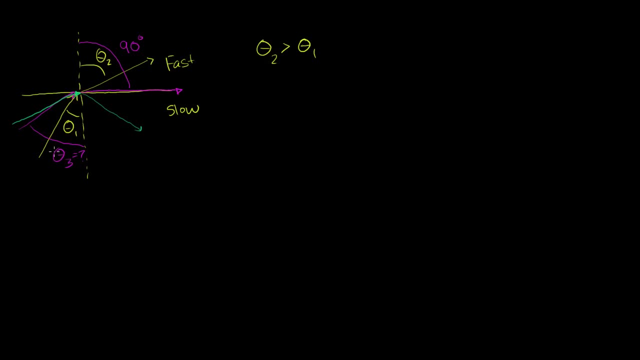 is going to be called our critical angle, because if you have an angle anything larger than that, then you're actually not going to have refraction, you're actually not going to escape the slow medium, you're just going to reflect at the boundary. 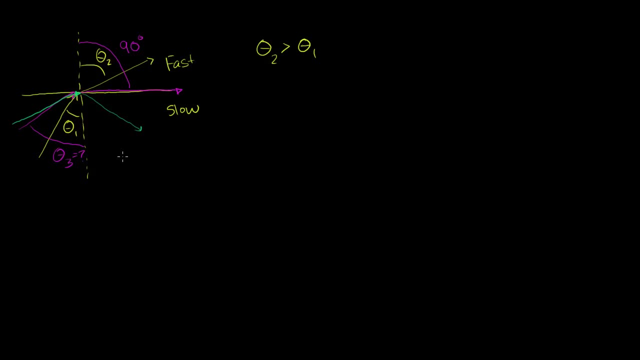 back into the slow medium. So let's try to figure that out, and I'll do it with an actual example. So let's say I have water. let's say I have, this is water. it has an index of refraction of 1.33,. 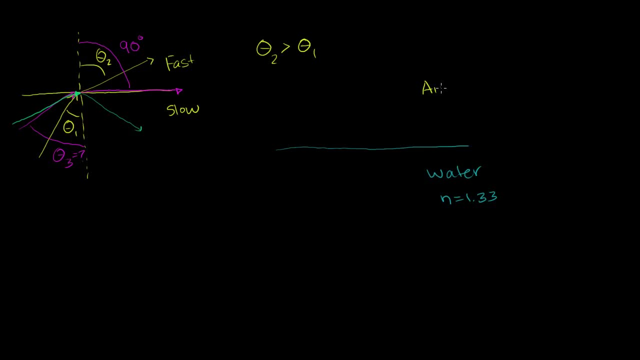 and let's say I have air up here and air is pretty darn close to a vacuum and you know we saw this index of refraction is 1.00029 or whatever. but let's just for the sake of simplicity, 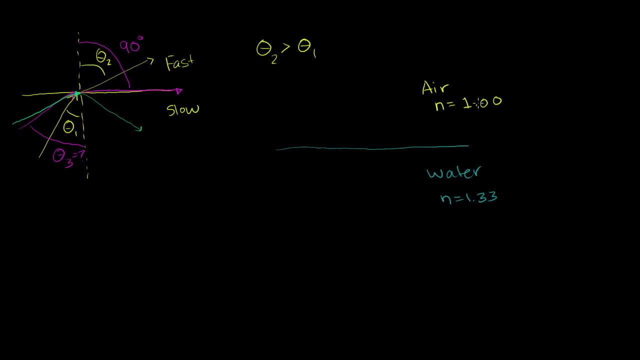 say, its index of refraction is 1.00.. And what I want to do for light? for light that's coming out of the water, for light that's coming out of the water, let me find another color for light that's coming out of the color. 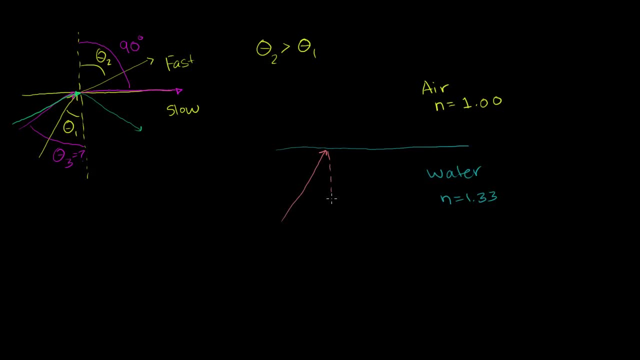 I want to find some critical angle, some critical angle- here I'll call it theta critical- where the angle of refraction, where the angle of refraction is 90 degrees, where it will actually never escape. so where this right over here? 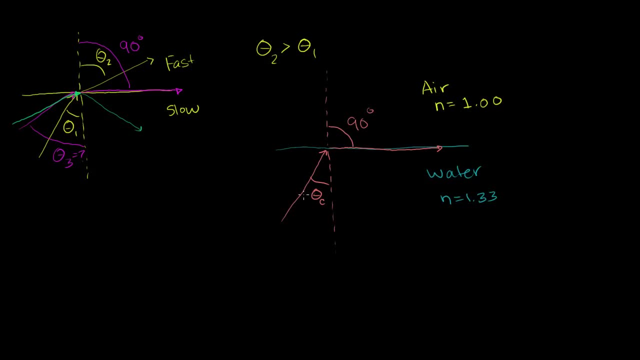 this is 90 degrees And so if I have any angle less, any incident angle less than this critical angle, I will escape. At that critical angle I just kind of travel at the surface, and anything larger than that critical angle I will actually reflect. 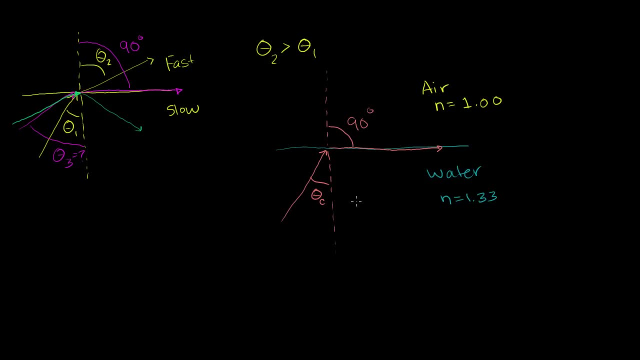 I'll actually have total internal reflection. So let's think about what this theta, this critical angle, could be. So we'll just break out Snell's Law again. We have the index of refraction of the water: 1.33,. 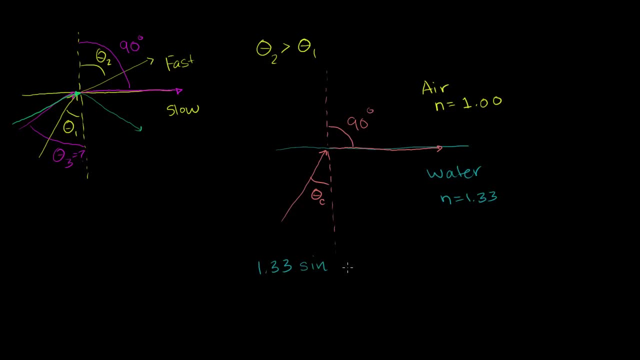 times the sine of our critical angle, times the sine of theta critical is going to be equal to the index of refraction of the air, which is just 1, times the sine of this refraction angle. so times the sine of 90 degrees. 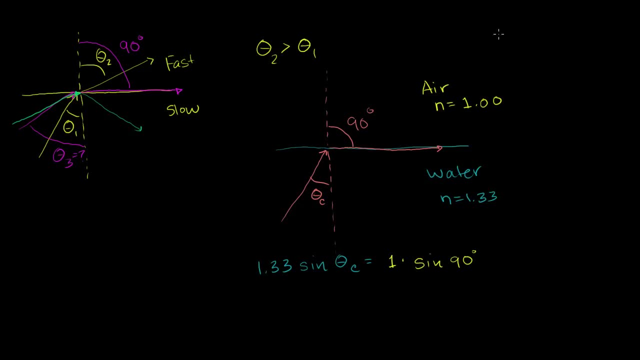 Now, what is the sine of 90 degrees? And to figure that out you have to think about the unit circle. You can't just do the SOHCAHTOA, because this is actually why the unit circle definition is useful. But if you think of the unit circle, 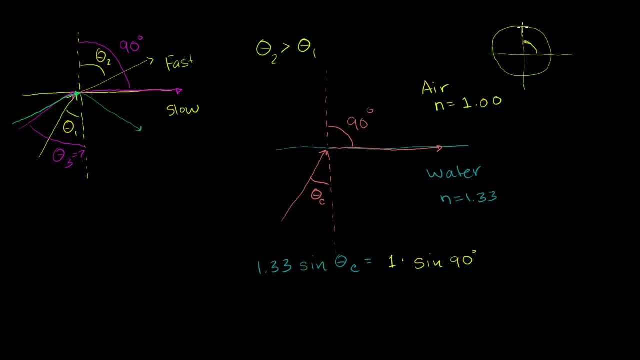 if you go 90 degrees. we are now here on the unit circle and the sine is the y-coordinate. So this is a unit circle, So that is a 1.. That's a 1 right over here, So the y-coordinate. 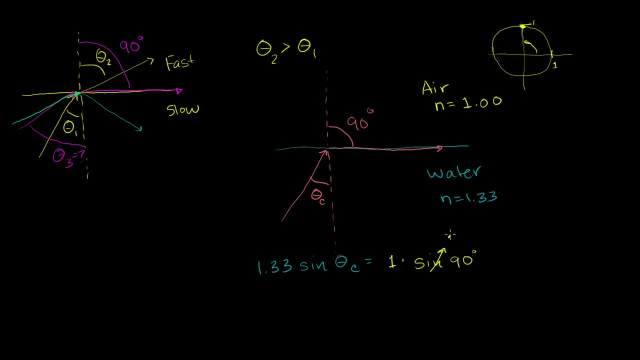 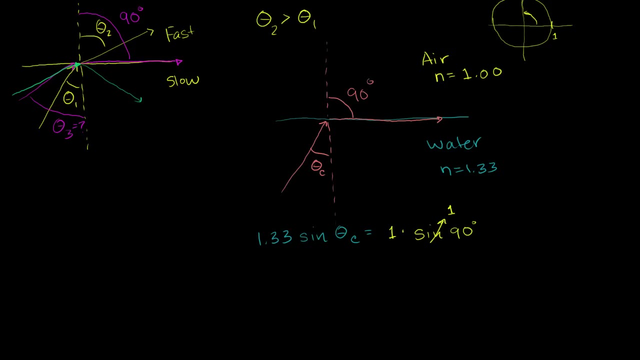 right over here is 1.. So this right over here is going to be 1.. So if we want to figure this out, we can just divide both sides by 1.33.. So we get the sine of our critical angle is going to be equal to. 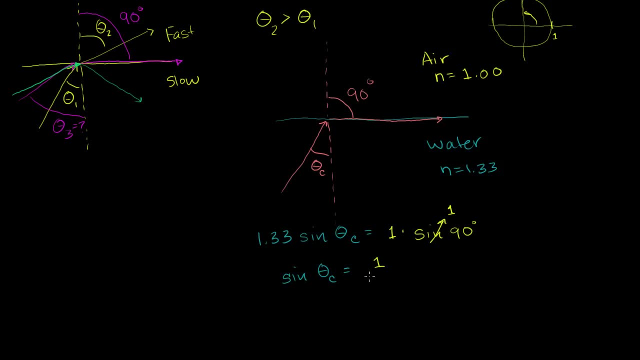 well, this is just 1, this is just going to be 1, over 1.33.. And if you wanted to generalize it, this is going to be the index of refraction. This, right here, is the index of refraction of the faster medium. 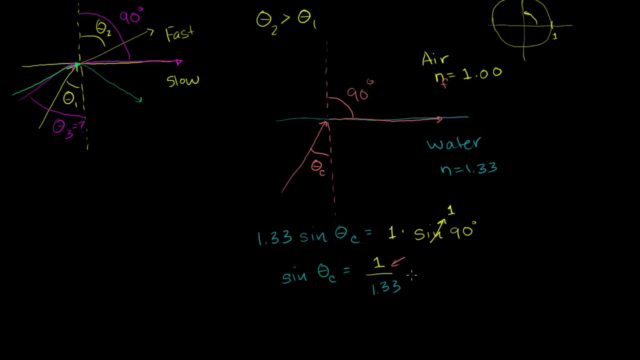 That right there we could call that index of refraction of the faster medium. And then this right here is the index of refraction of the slower medium. I'll call that the slower medium, So that right there is ns, And because you're always going to find the sine of 90 degrees. 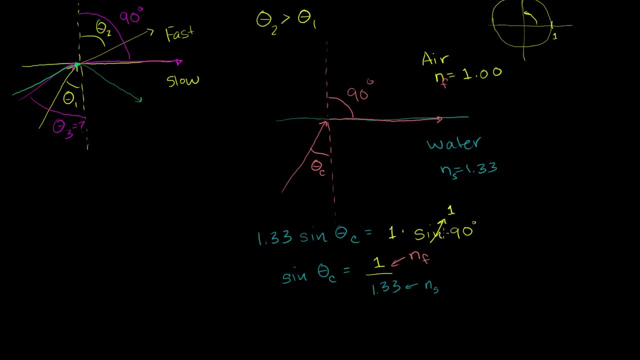 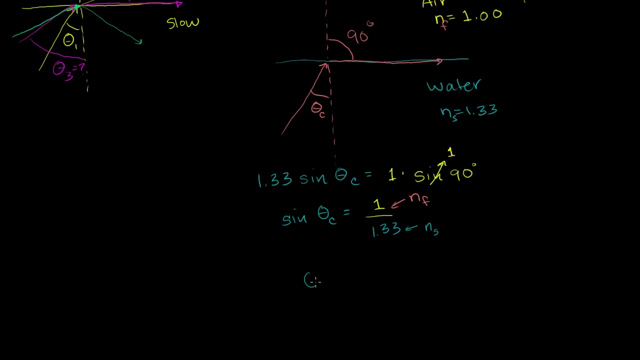 this is always going to simplify to 1 when you're finding that critical angle. So just to keep solving it, before we get our calculator out, we could take the inverse sine of both sides and we get our critical angle. Our critical angle is going to be the inverse sine. 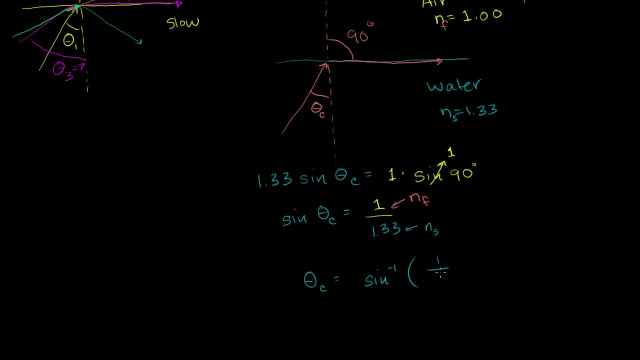 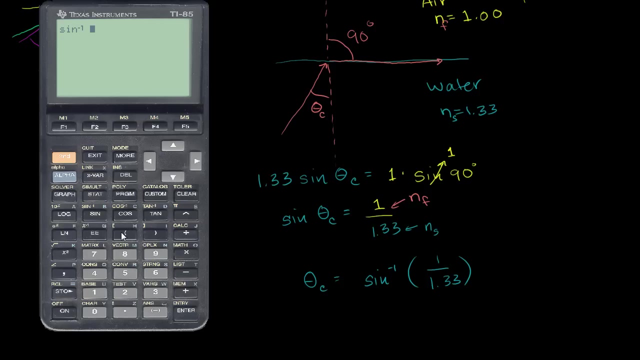 the inverse sine of 1 over 1.33.. And we can just get our handy TI-85 out again. Let's get the TI-85 out, And so we just want to find the inverse sine of 1 divided by 1.33.. 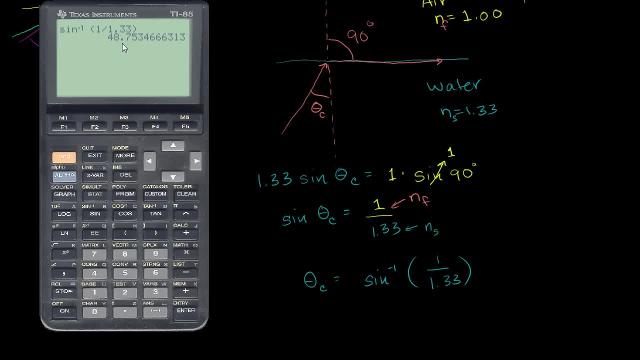 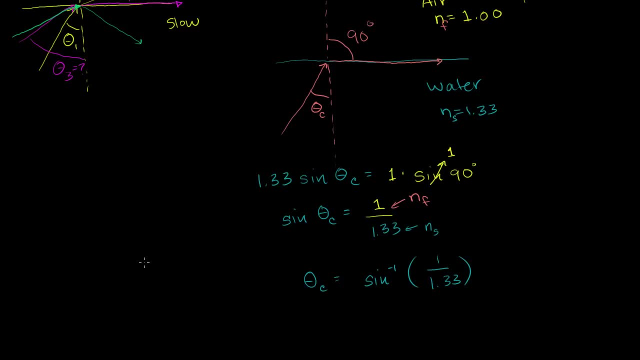 And we get 48 point. we'll just leave it at 48.8 degrees. So this right here. so our critical angle, our critical angle is 48.8 degrees, which tells us. so this right here is 48.8 degrees. 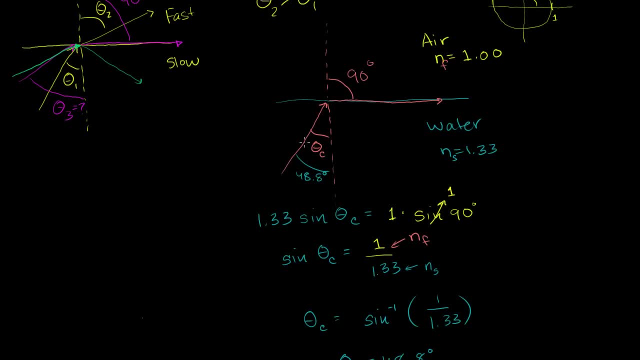 which tells us if we have light leaving water at an incident angle of more than 48.8 degrees, at more than 48.8 degrees, it actually won't even be able to refract. It actually won't be able to escape in the air. 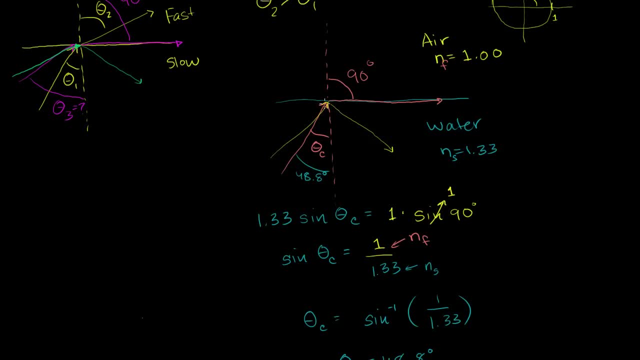 It's actually just going to. it's actually just going to reflect at that boundary. If you have angles less than 48.8 degrees it will refract. So if you have an angle right over there, it will be able to escape and refract a little bit. 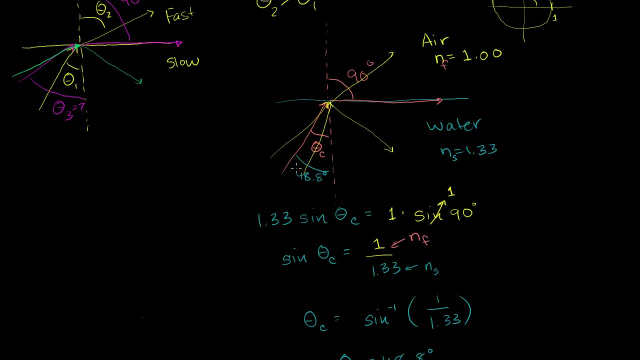 And then right at 48.8, and this is- I've rounded it a little bit, but right at that critical angle, you're just going to travel, you're going to have a refraction angle at 90 degrees or really just travel at the surface of the water. 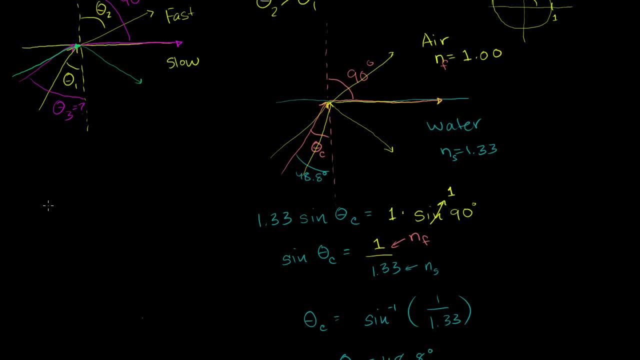 And this is actually how fiber optic cables work. Fiber optic cables are just, you can just, they're just. you can almost just view them as kind of glass pipes And the light is traveling. The angle of the incident, angles are so large here. 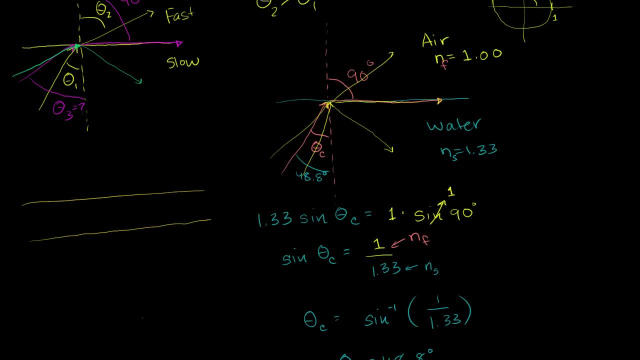 that the light will just keep reflecting within the fiber optic. So this is the light ray. They travel at larger than the critical angle. So, instead of escaping, instead of escaping into the surrounding air or whatever, it'll just keep reflecting within the glass tube. 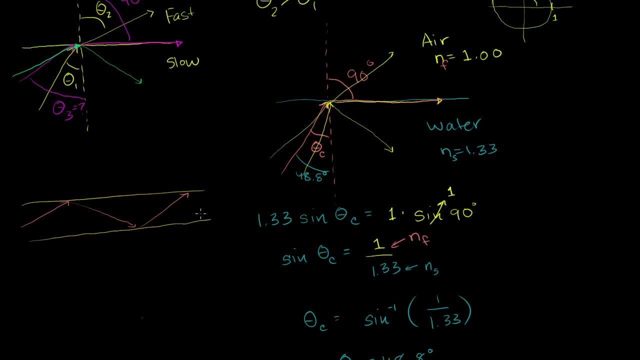 within the glass tube, allowing that light information to actually travel. So anyway, hopefully you found that reasonably interesting. 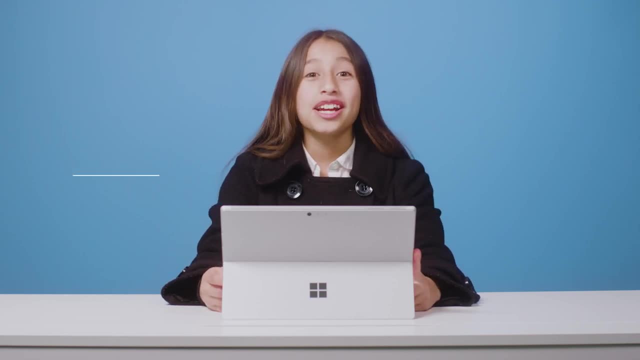 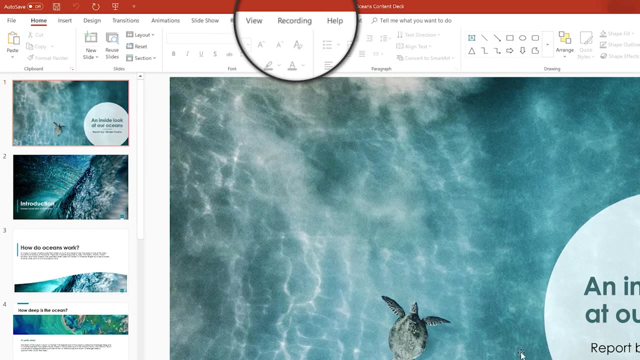 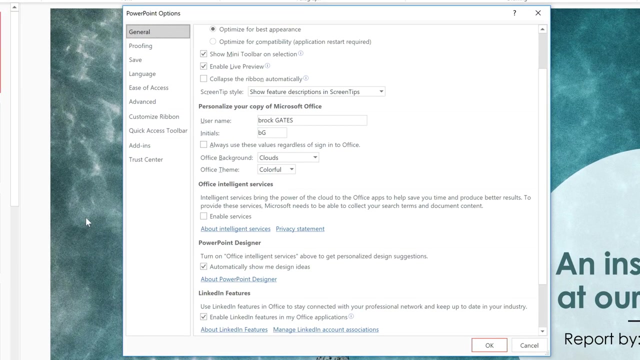 Hi everyone. I'm Eileen and I'm in sixth grade. Today we are going to learn how you can narrate your PowerPoint videos, So let's get started. Make sure you can see the record tab by clicking file, then options. Then choose customize ribbon and. 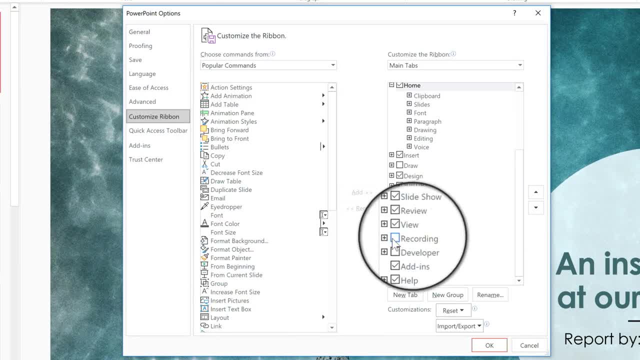 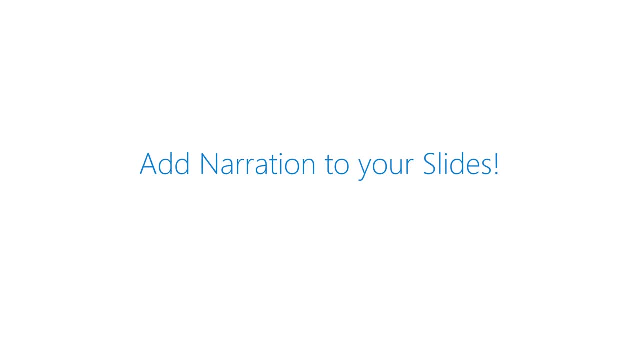 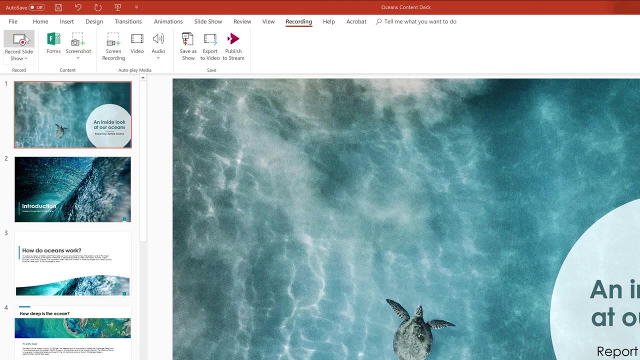 check the box next to recording. Click OK in the dialog box and your recording tab will appear in PowerPoint. Now it's time to add narration to your slides. Click your recording tab and select record slideshow. You'll see options for recording audio and video as well. You'll also see tools for using digital inking. 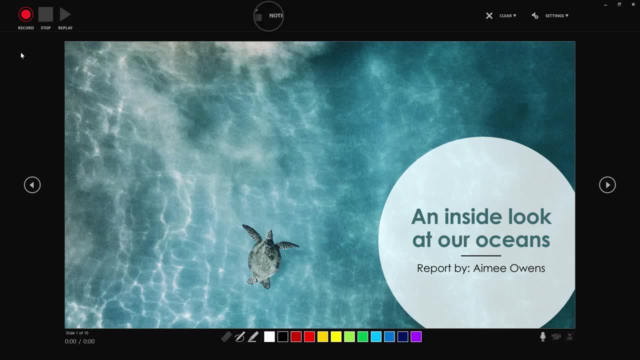 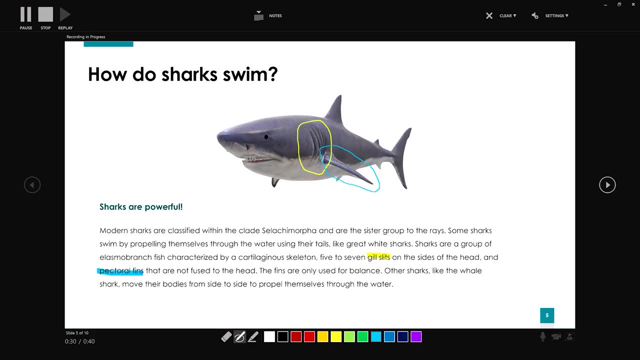 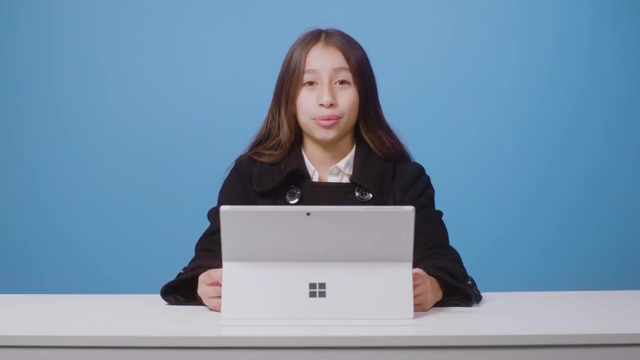 while you talk. If you have notes embedded in your PowerPoint, they'll appear at the top. When you're ready, click the record button. When you're done recording, hit stop and review your work. Okay, time to turn your narrated PowerPoint into a video. There are two ways to do this.